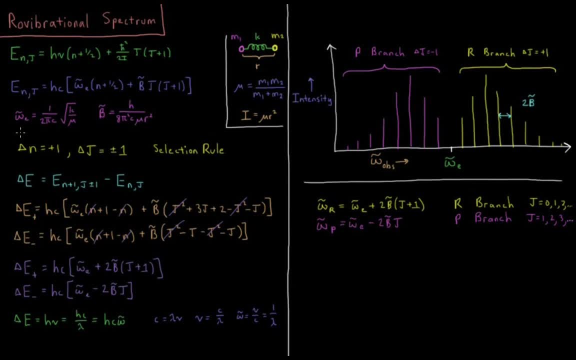 The selection rule is that delta n- the change in our vibrational energy level- is plus one. so we're absorbing a photon- this is an absorption spectrum- And delta j- change in our rotational energy level- can be plus or minus one. 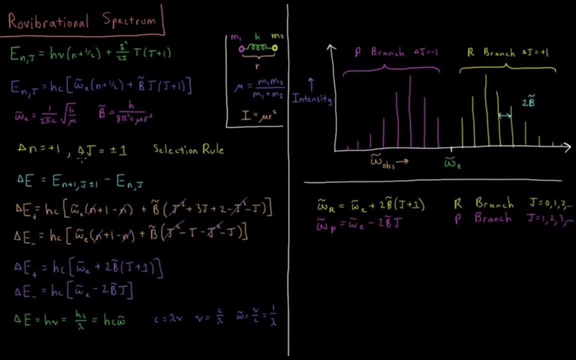 Remember that our vibrational energy levels are much, much bigger than our rotational energy levels, so this is always going to be a positive result. So delta e is going to equal e of n plus one j plus or minus one minus e n, j accounting. 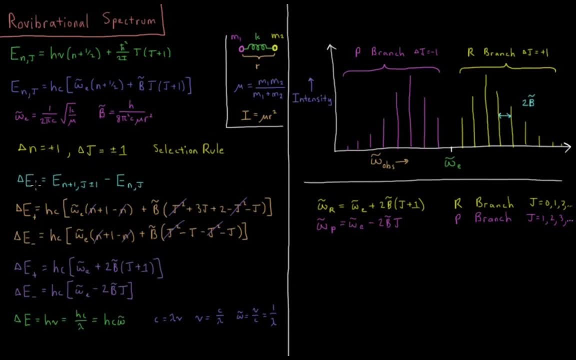 for these selection rules. So we have two different cases here, One where delta j equals one, One where it's minus one, And we'll look at delta e plus and delta e minus. So delta e plus equals hc, omega e n plus one minus n. 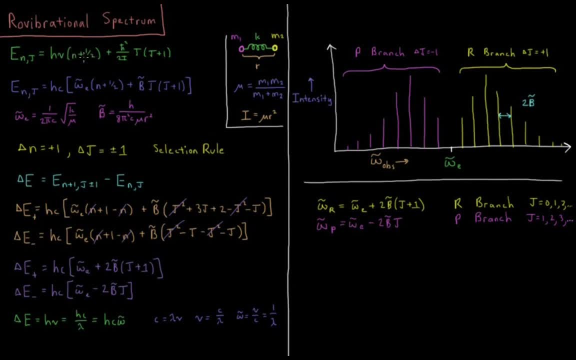 So we have n plus one plus one half, minus n plus one half. So that gives us the value that results down. here We're left with an omega e. there. Same case in delta: e minus For the vibrational part. we just get an omega e. 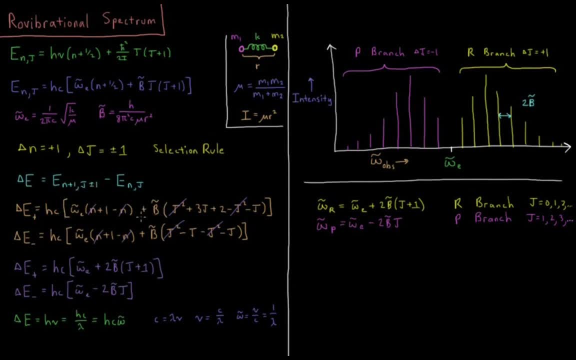 Plus b bar, and we substitute n, j plus one and then subtract j For the quantity j times j plus one. So j squared plus three, j plus two Or j plus one. time j plus two Minus j times j plus one is minus. j squared minus j. 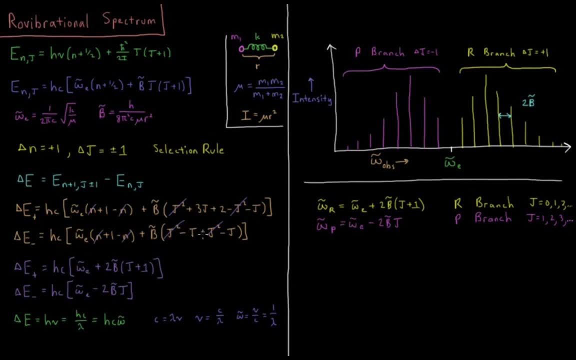 In e minus, we have j squared minus j minus j squared minus j. So what we have is j times j minus j. That equals delta j j squared minus j minus e minus. And e minus equals j squared minus j minus j squared minus j. Safari d squared minus. 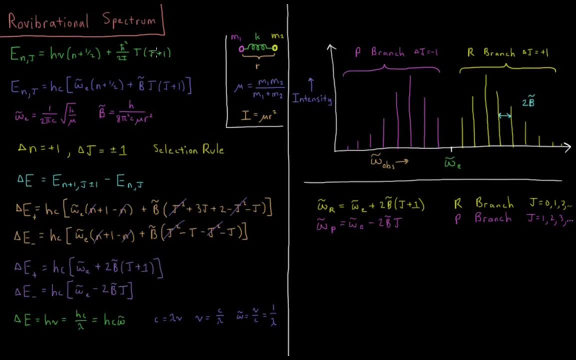 plus 1 times j, minus 1 times j. So the j squareds cancel. in each case We have 3j plus 2 minus j is 2j plus 2.. So we have, and we have a minus j minus j, just a minus 2j there. So for delta e plus we. 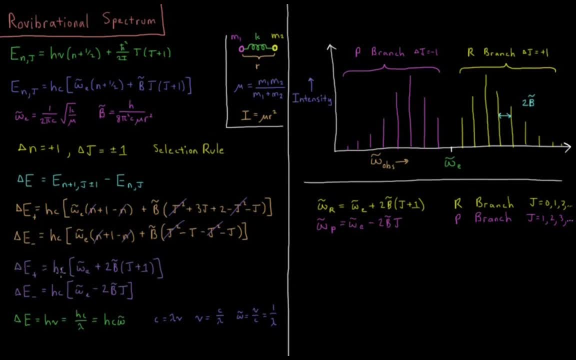 have: e equals delta, e plus equals hc. omega e plus 2 b bar times j plus 1.. Delta e minus equals hc, omega e bar minus 2 b bar times j. So the energy of our transition is equal to Planck's constant times the frequency of the photon we're going to absorb. Speed of light equals wavelength times. 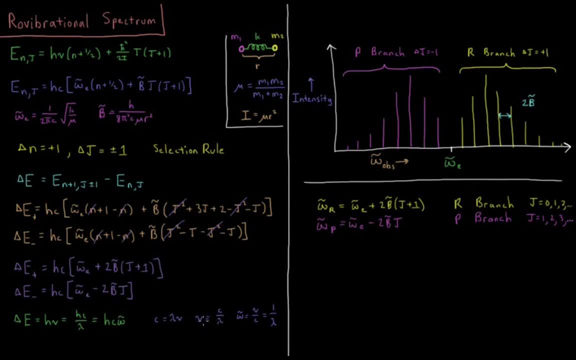 the frequency of that photon. Frequency equals speed of light over wavelength. So inverse wavelength 1 over lambda is equal to the frequency divided by speed of light. So we're taking our energy and we're dividing it by the frequency of light. So we're taking our energy and we're dividing it. 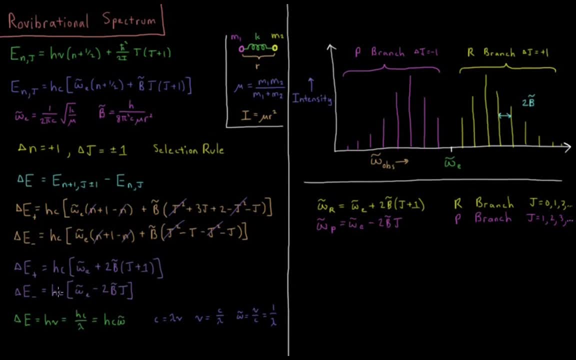 it by hc to get the value in wave numbers. so delta e equals hc omega observed or omega bar observed. so this delta e plus and delta e minus gives us two different cases. this case is going to be what we call our, our fundamental transition, plus some energy time, and the minus case is 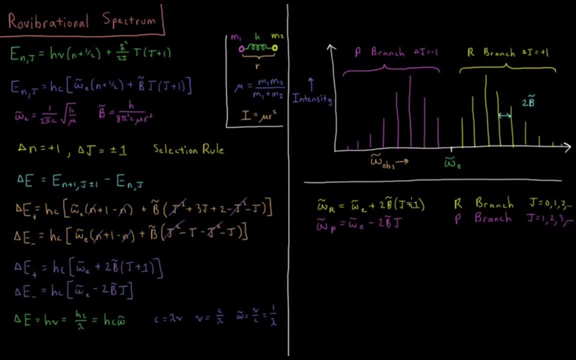 the fundamental transition minus some energy. so what we get is two distinct branches: one, the r branch, where the increase we increase above the vibrational transition omega, e one, the p branch, where we are less than the vibrational transition energy. so what we get is this kind of double wing. 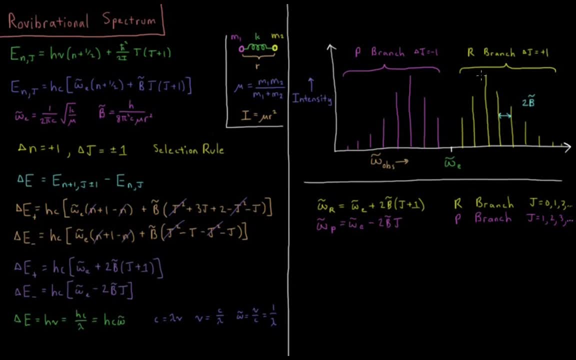 shaped spectrum here and this is based off of what the occupation of rotational states is at room temperature. so the shape of this actually comes from statistical mechanics. some of you might look into that in your stat mech or, if you go more heavy into spectroscopy. some of you'll look into that, some of you won't. but the shape of this comes from the fact of 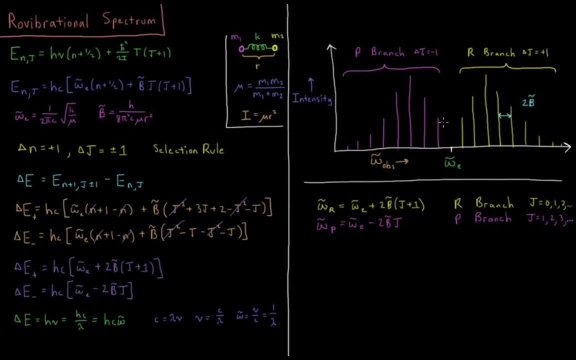 how the energy levels are separated and what the degeneracies of the energy levels are. so here this is a transition from j equals zero to j equals one, j equals one to j equals two, two to three, three to four, four to five, et cetera. and here we have the transition from j equals one to j equals zero.